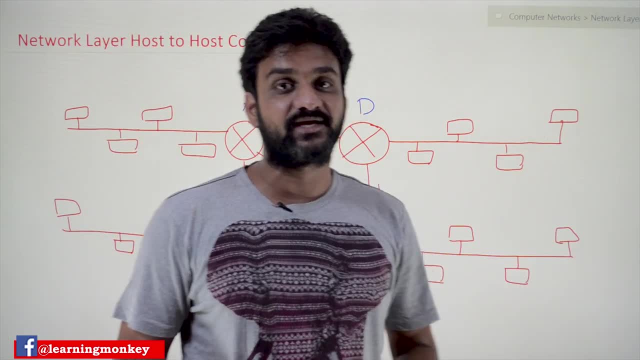 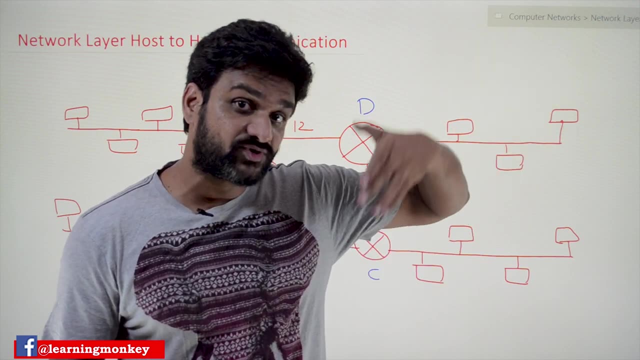 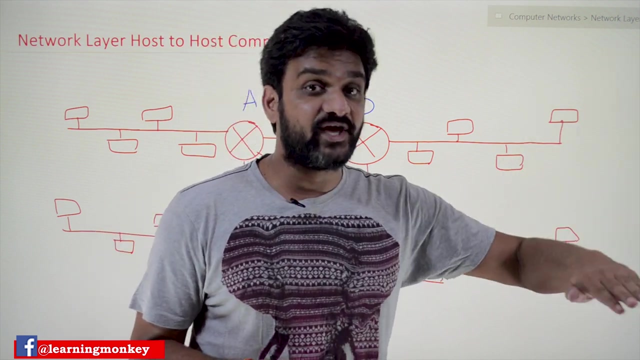 In the previous section where we have discussed about data link layer. there we said that the data link layer is called as node to node communication. The communication that is going to happen in the data link layer is called as node to node communication. In the same way, the network layer is called as host to host communication. 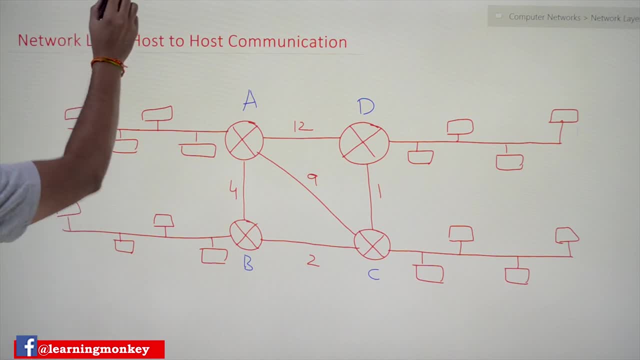 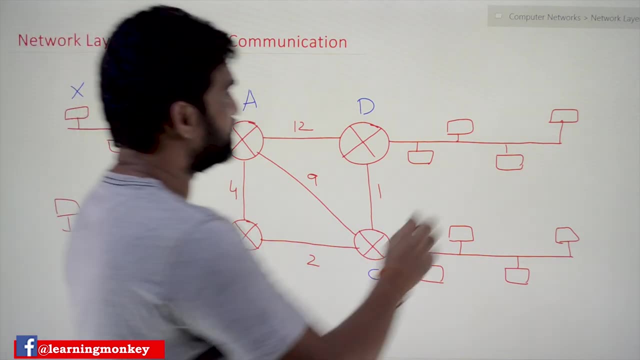 Why it is called as host to host communication is, for example, for example, this system: name it as X. This system wants to communicate with this system Y. So how the communication is done and what is the role played by the network layer. 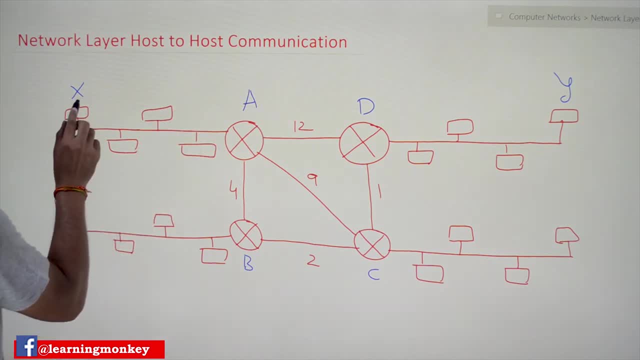 So, with that concept, we will try to understand. So first, what happens is this: X will send the packet that needs to be delivered, The data that needs to be delivered. that packet will be transferred to A, because this is the default router to which the system to which the data has to be transmitted. 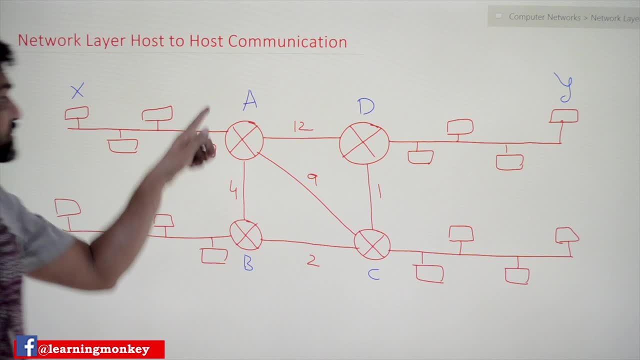 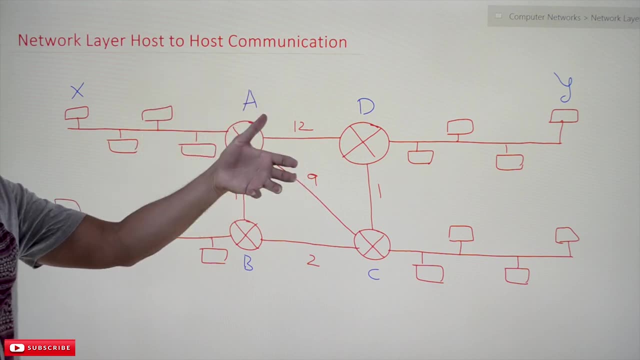 if it has to cross the network. If the communication is within the network, then both those systems will get communicated. If the communication is out of the network, the packet that has been that needs to be sent will be transferred directly to the node which is directly connected. 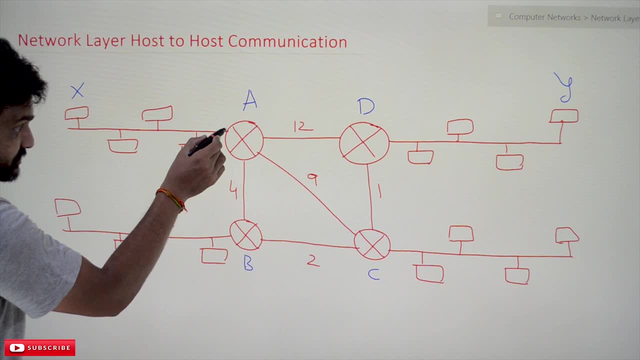 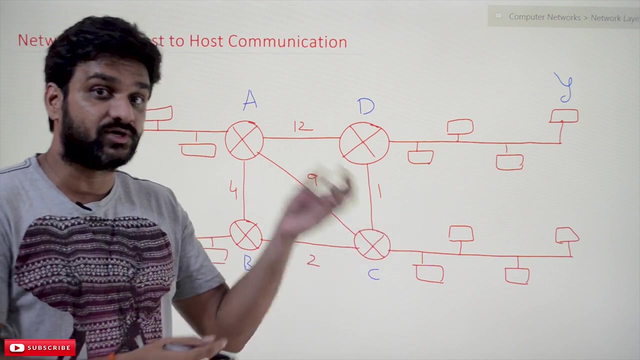 So that is the reason why the data link layer, so the objective of the data link layer, is called as node to node communication. So node to node, So the details that are there in the frame are used to communicate from one node to another node. 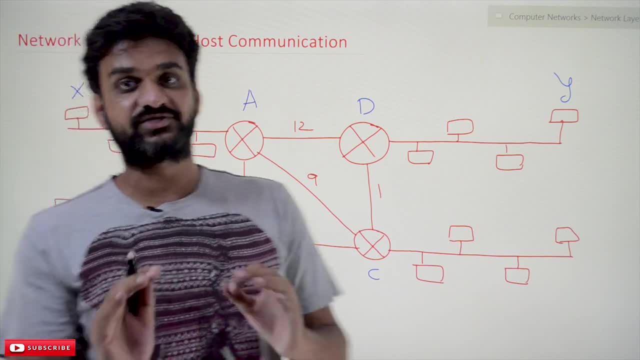 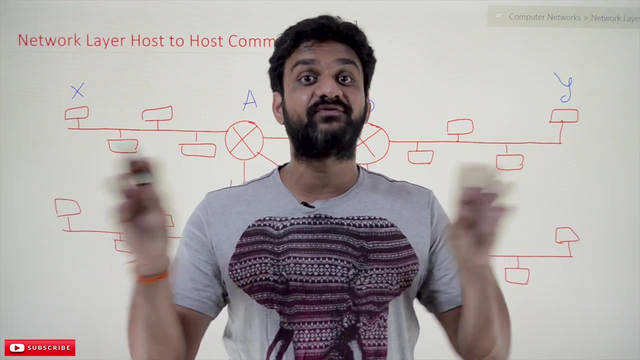 So what is the difference between host and node? First of all, we have to get the clarity. Host means the two systems which are participating, which wants to communicate with each other. they are called as host. And what is meant by a node? 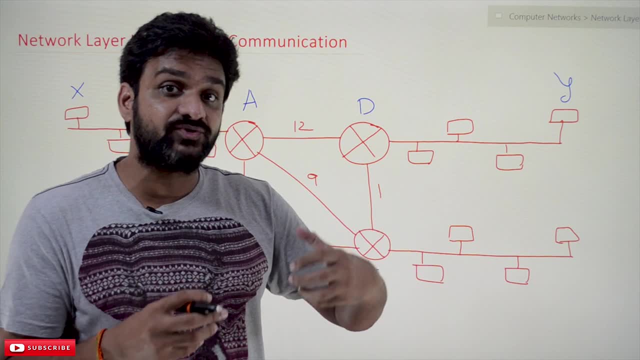 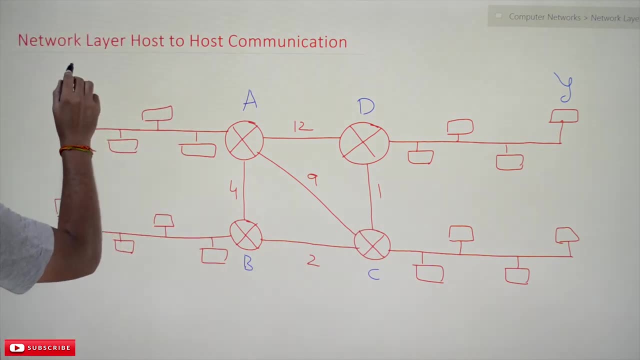 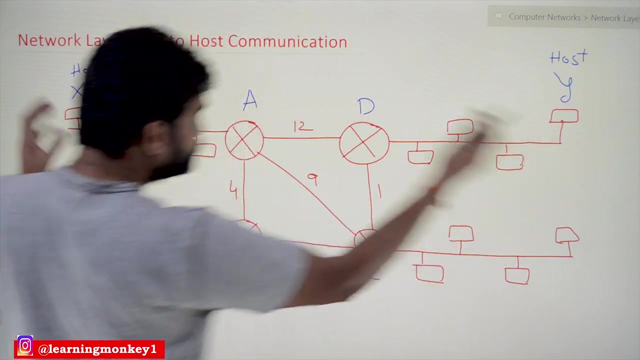 Node means an intermediary device which helps us to make the communication possible, So that is what we call it as node. So here the host, or X is a host, This is a host and the other one is the Y is a host, Because these are the two systems which wants to communicate with each other? 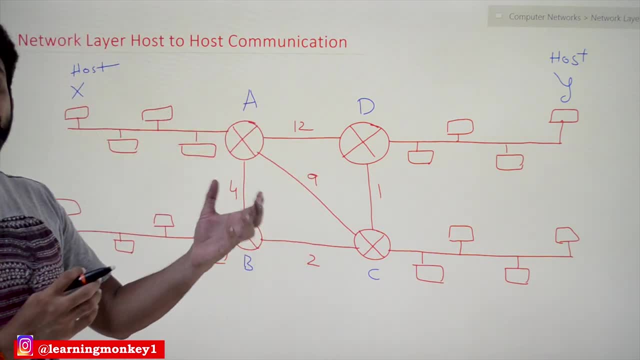 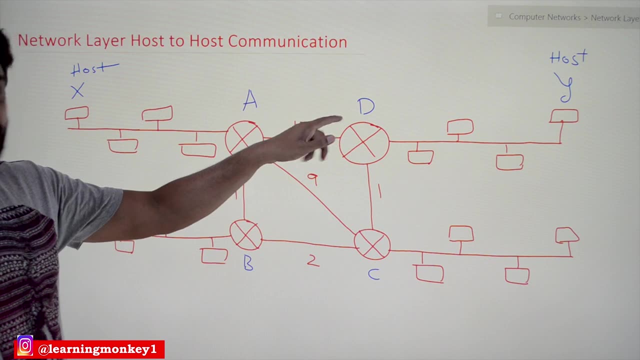 Who are all the devices which are helping us to make that communication possible? So the first one is the devices, or this one, this one, A, B, C, D, the routers. All these four routers are the nodes which make the communication possible. 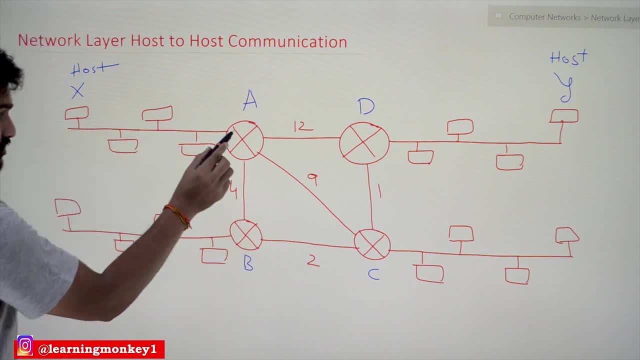 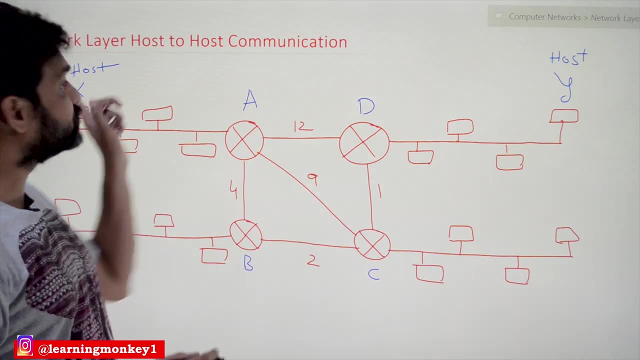 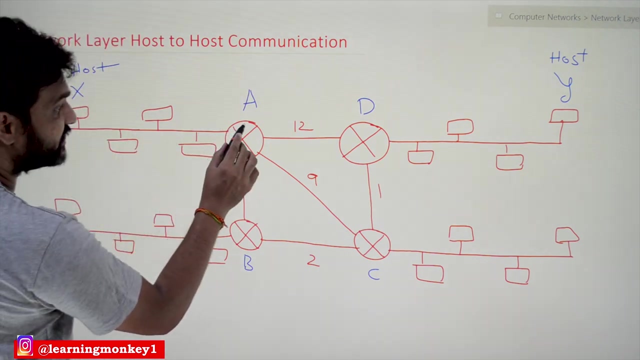 Okay, And the communication from one node to another node is managed by data link layer And the communication from one host to another host is all managed by network layer. So how that happens. So, once the packet has been received at the router, what the router will do. 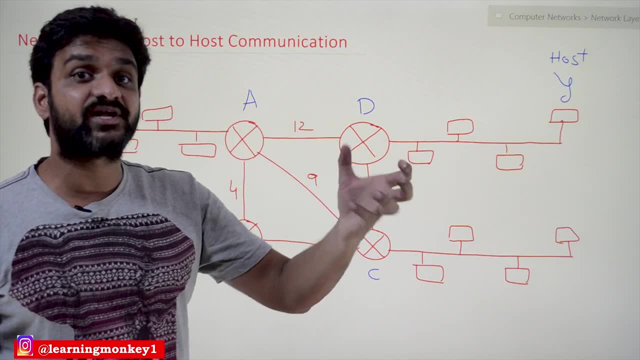 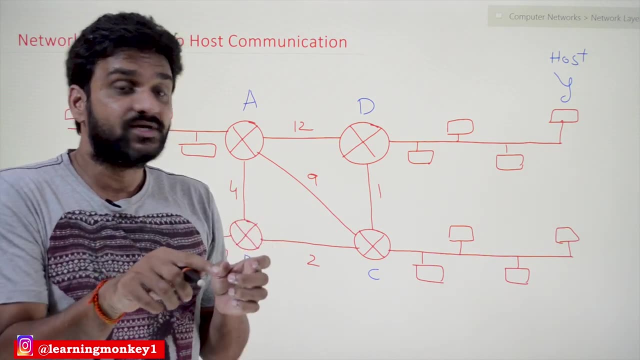 So where the router is? router is a network layer device. So what is the duty of the router? It is going to transfer the packet to the interface. So it is having three different interfaces, So it will transfer the packet to one of those interfaces. 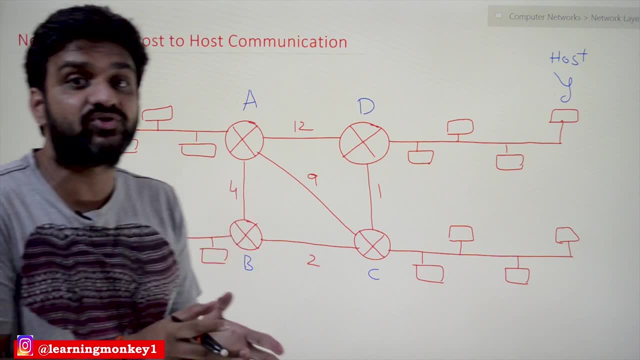 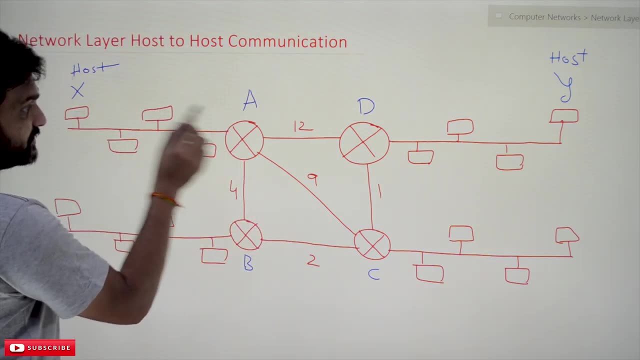 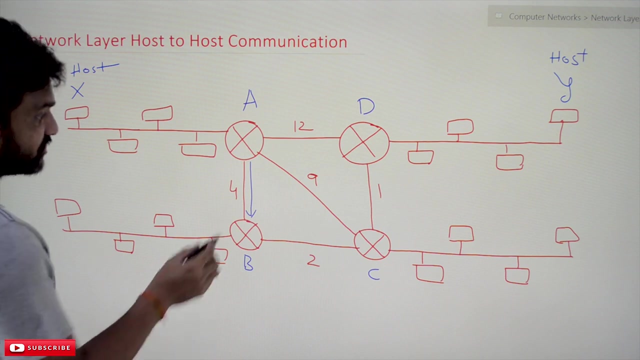 So that it will take the shortest amount of distance. So in our case, the packet from X will be transferred to A And from A it will get transferred through this interface Because the shortest path from A to D is 4.. This is the shortest path. 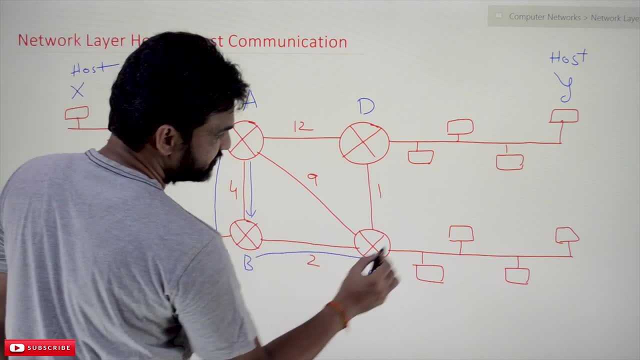 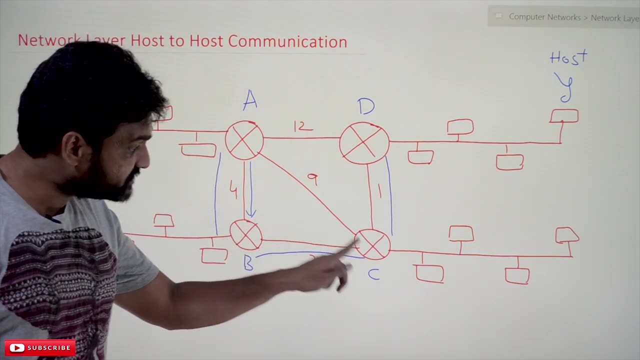 So all these concepts we have discussed in our previous videos, So the entire concepts of network layer has already been discussed. So the communication is from this node to another node And from this node to this node And from here it will get transferred to this node. 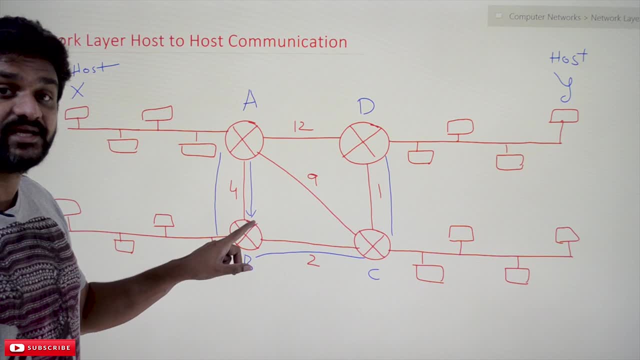 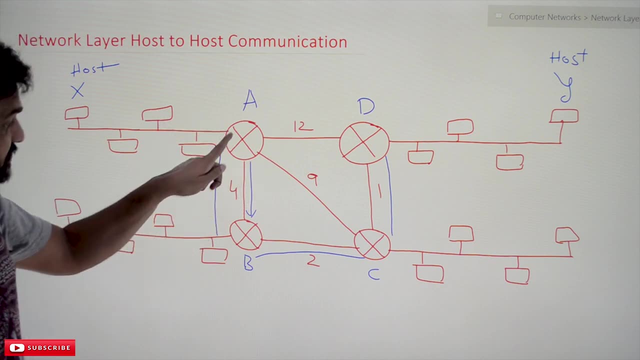 So in between, so from node to node, it is what we call it as data link layer. So here it is: Ethernet Ethernet. in Ethernet the data link frame is used for communication. This is a point to point communication. So from here it will get transferred to this point. 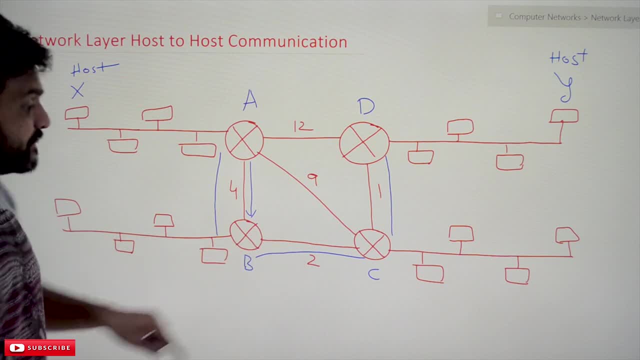 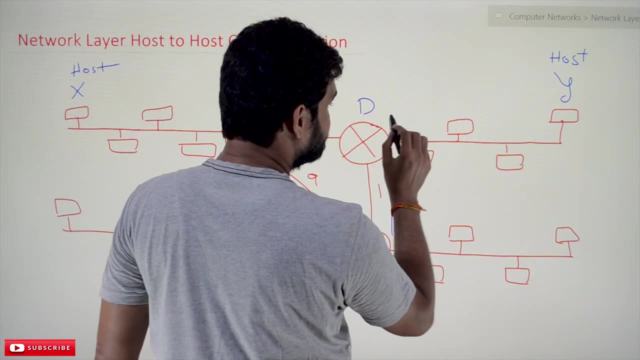 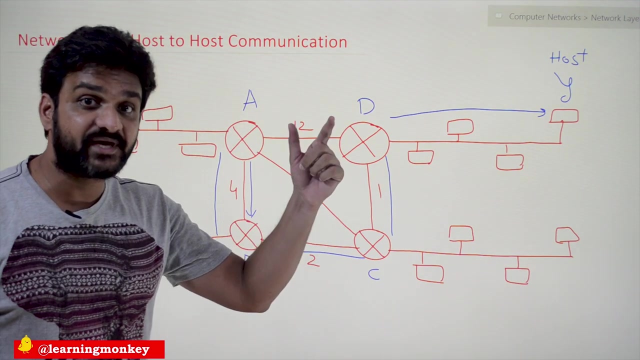 And from here to here it will get transferred to this point. Okay, So this is the next node: From here it will get transferred to here, And from D It will finally get transferred to Y. and who is helping us to identify the next node? who is helping us? 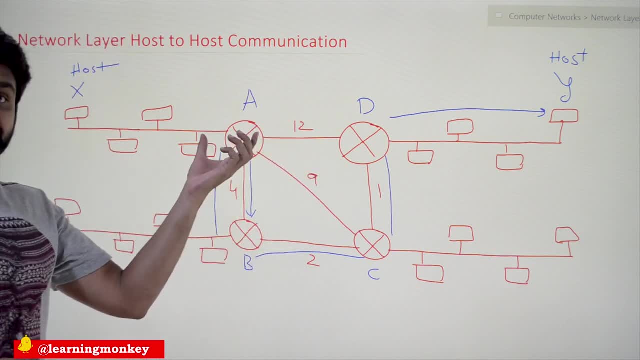 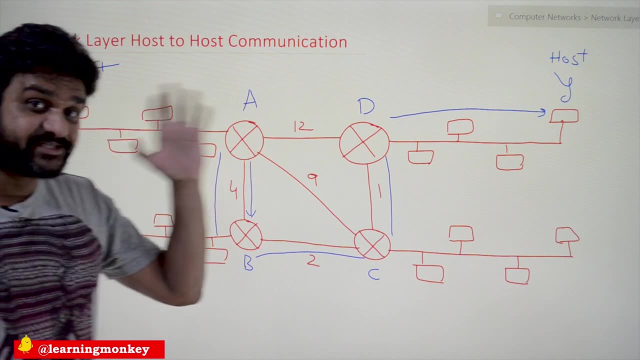 So this point is very important. who is helping us? It is the router. We were able to decide one of the interface from all the interfaces which are connected, So that decision is made by the routing algorithms and the routing table, which is which is getting generated on the router.